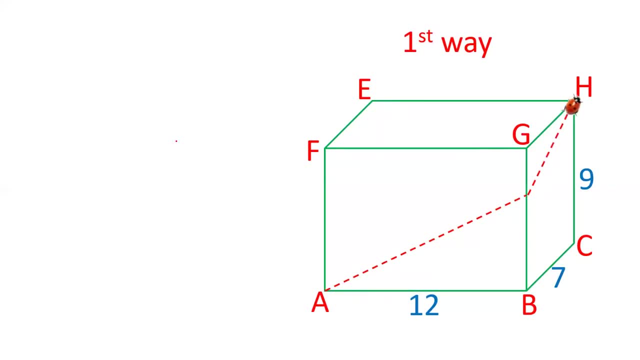 move up to H. This is the shortest. Let us see what is this distance Basically? this is the front face and this is the side wall. Front face is 12 by 9.. Side wall is 7 by 9.. So this length is hypotenuse of this right angle triangle. 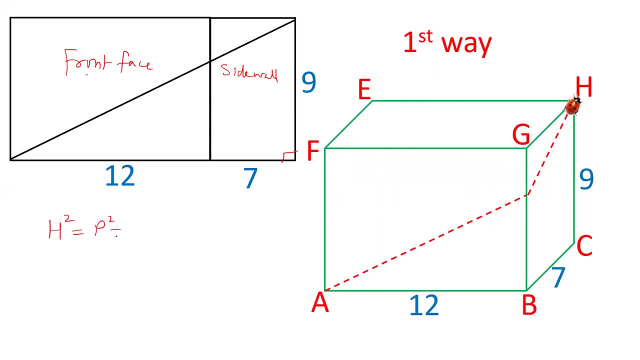 So let us calculate the length: H square is equal to P square plus B square. Perpendicular is 9.. Base is 12 plus 7,, 19.. 12 plus 7, 19.. 81 plus 361.. That gives us 1, 1 and 2,, 36 and 8, 44.. 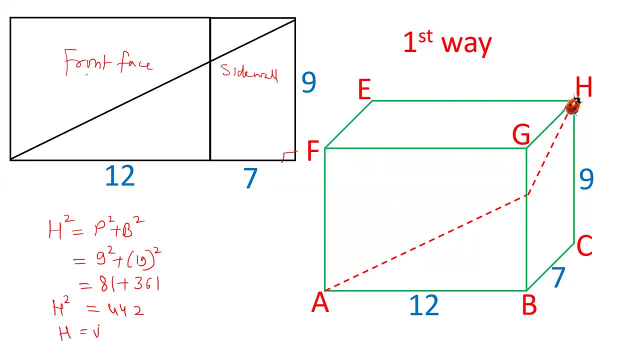 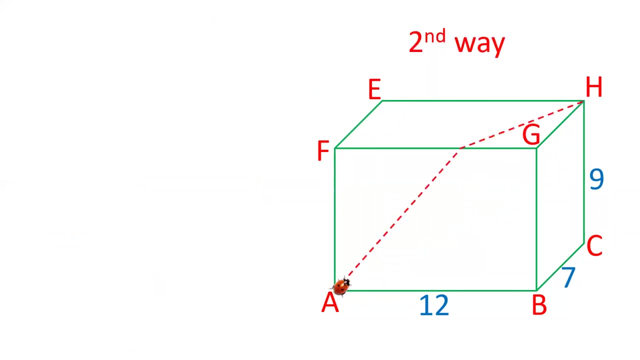 And H, square H is under root 4, 42,, which is approximately 21.01 maybe. So this length is 21.01.. Now let us see. This is the second way it can reach. First, it can move this point, this along this line. 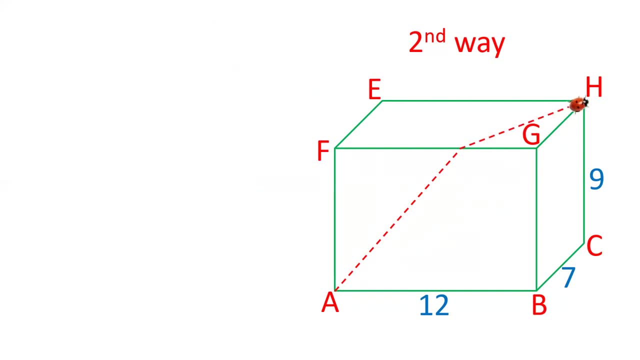 and then on the top surface, What is this length? This is the front face And this is the top face. It can move along. it has moved along this path. This is 12.. The top face is this one: 9 plus 7.. 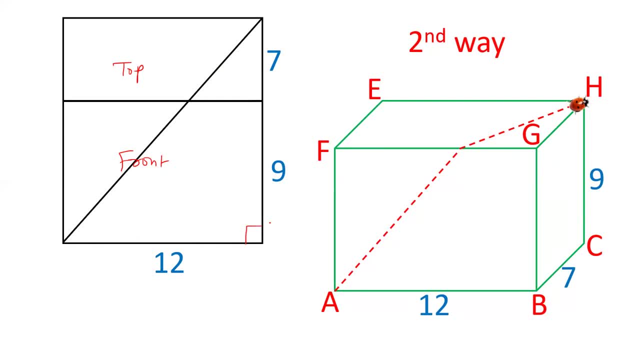 So again, this is a right angle triangle of side 12 and 9 plus 7.. So the length will be: h square is equals to p square plus b square. Perpendicular is 9 plus 7, 16 square and 12 square. 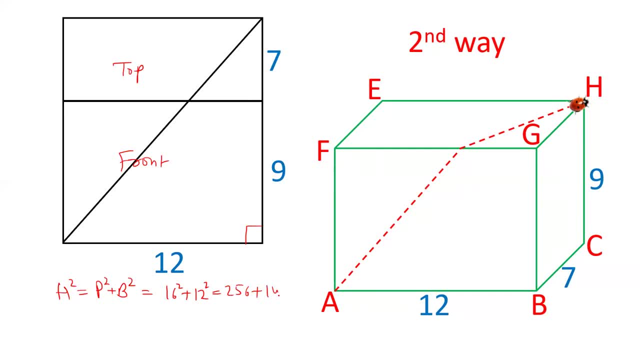 16 square is 256, 12 square is 144,, total is 400.. So this hypotenuse is, under root, 400, which is 20.. So, friends, the last one was 21 when it moved along this and then side wall, and this one is 20..